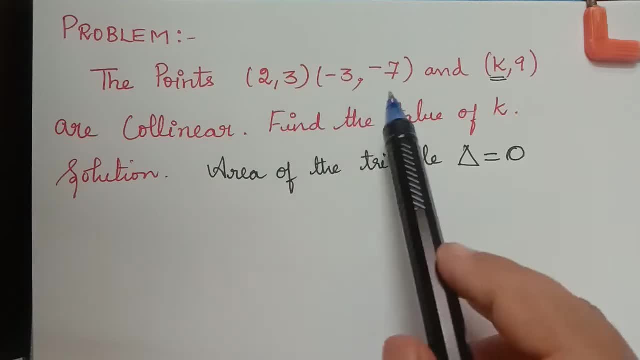 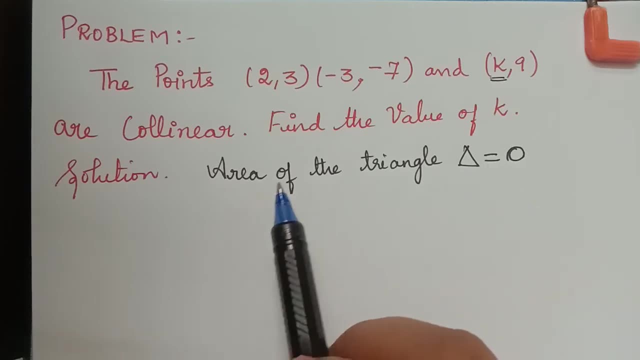 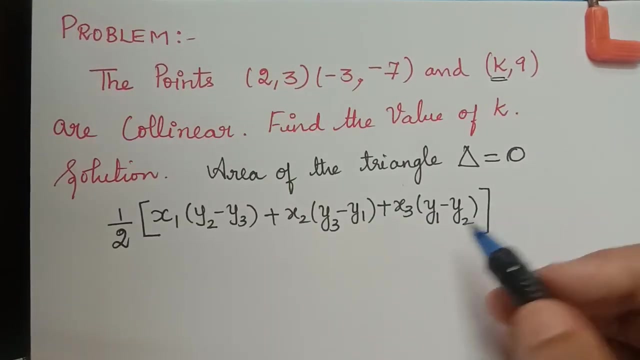 to be collinear. Now, here it is given that these three points are collinear and therefore the area of the triangle will be equal to 0, and area of the triangle is given by the formula. so it is given by this formula, and here we have the area of the triangle to be equal to 0, and so we can equate. 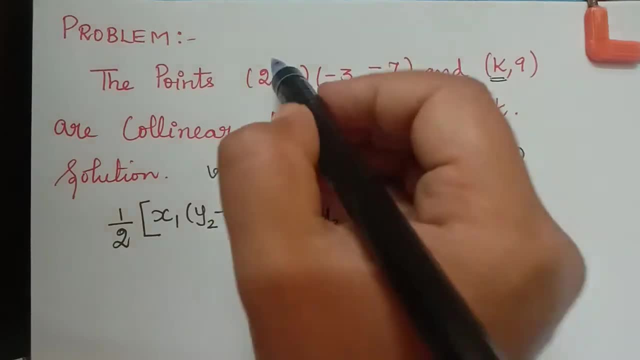 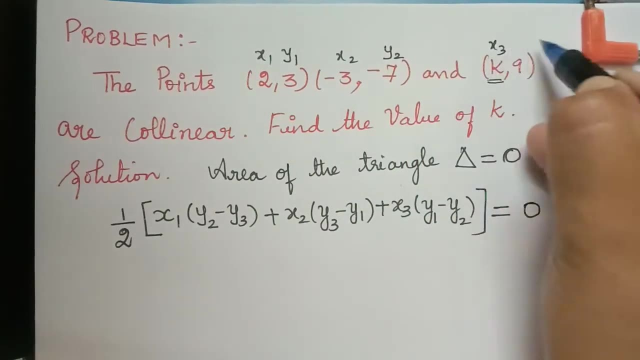 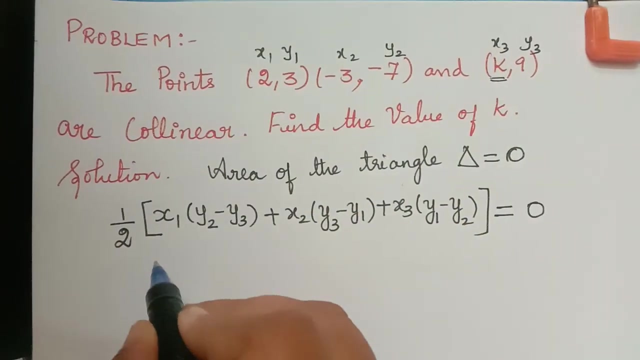 this formula to be equal to 0.. Now here, this is x1- y1, this is x2, y2 and this is x3- y3.. Now we shall substitute each of these coordinates in this formula, so we obtain 1 by 2 of what is x1 it is. 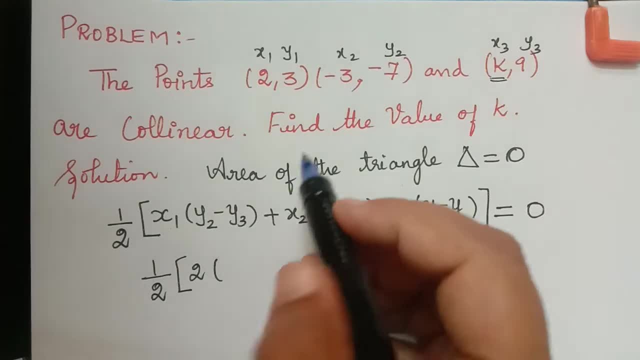 multiplied with y2 minus y3.. y2 is minus 7 minus y3, is minus 1 minus y3 minus y3 is minus 4 minus 6.. So it is actually a greater than just 1 pi minus 7, as evident. 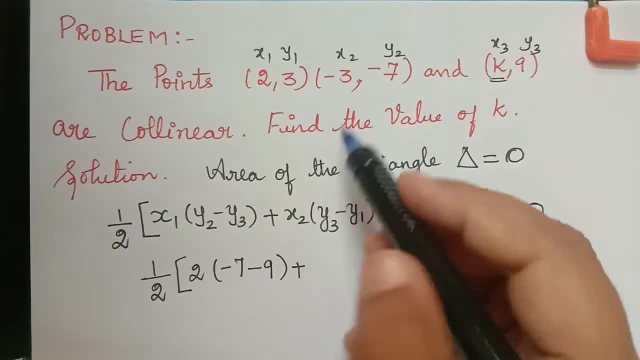 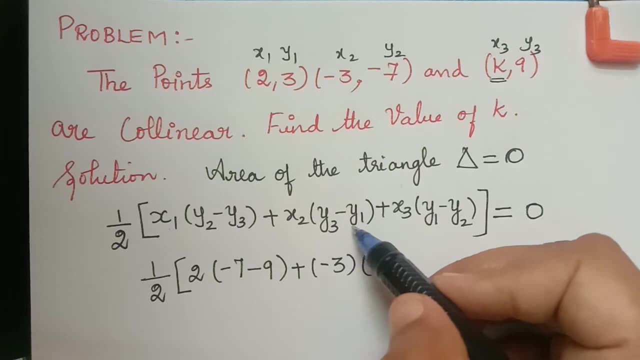 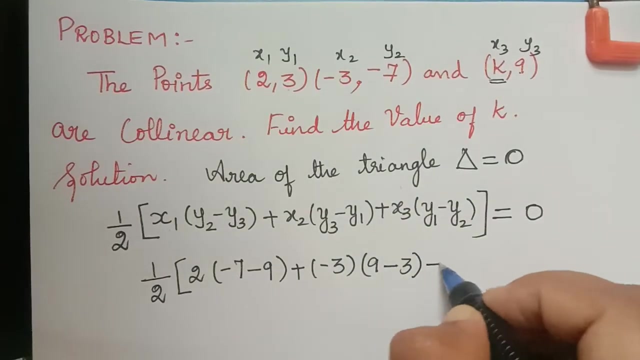 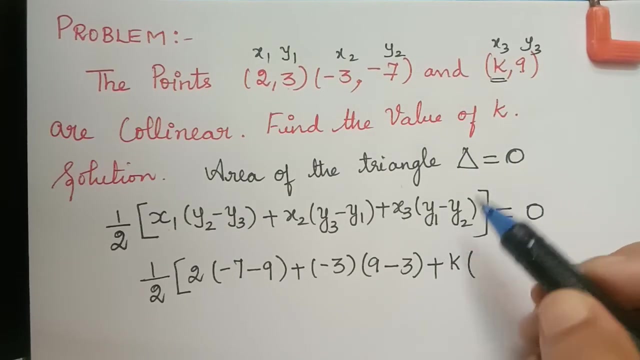 minus 9 plus x2, what is x2? it is minus 3. so we have to write: minus 3 multiplied with y3 minus y1, what is y3? it is 9 minus y1 is 3 plus x3, x3 is k. so k multiplied with y1 minus y2, y1 is 3. 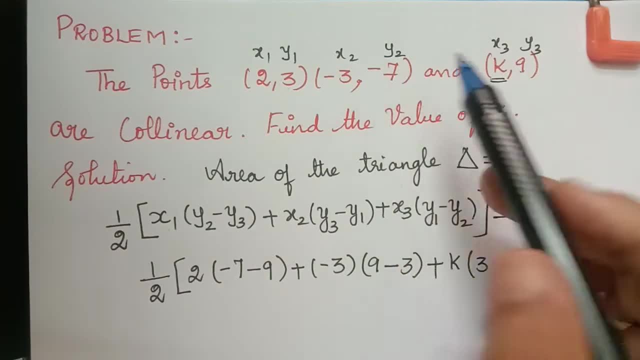 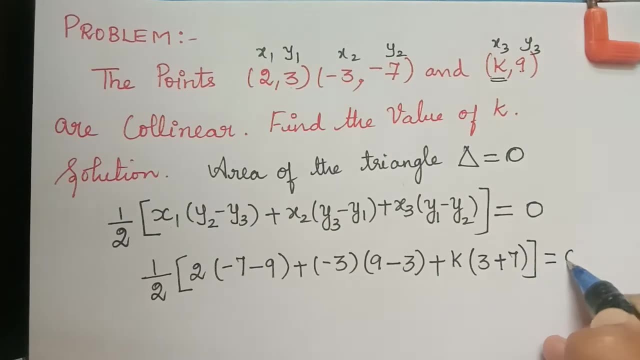 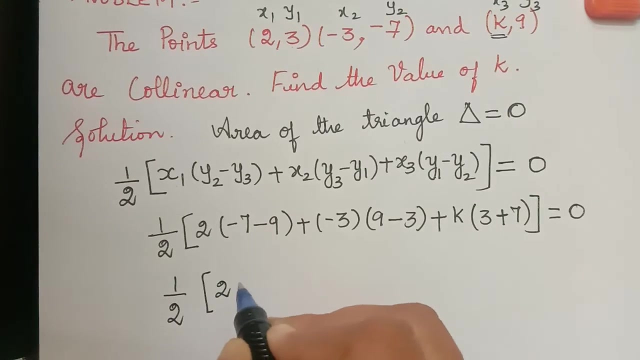 minus y2 is minus 7, so minus of minus 7 will become plus 7. okay, so this is equal to 0 and so, simplifying this, we obtain 1 by 2 of 2 multiplied with minus 7. minus 9 is minus 16, so 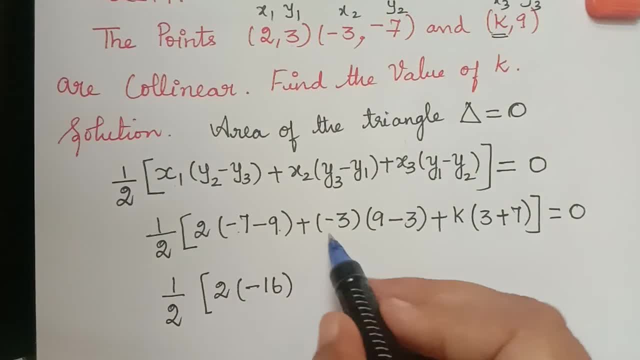 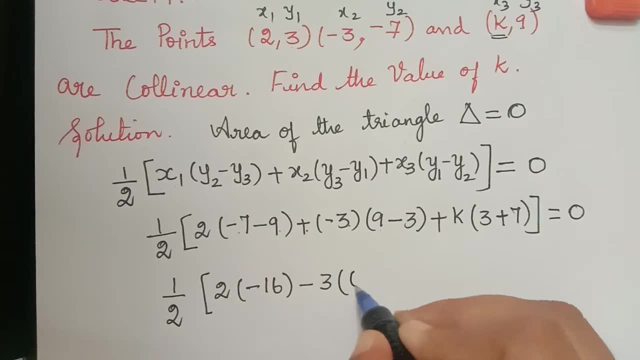 we have to add both and we have to write the negative sign, and here, plus into minus, is minus 3.. multiplied with 9 minus 3, which is 6 plus k, multiplied with 3 plus 7 is 10, is equal to 0.. 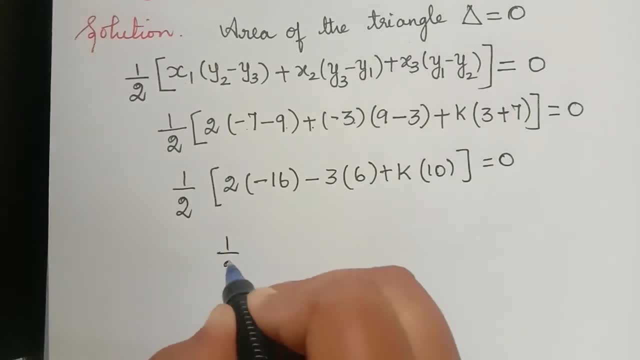 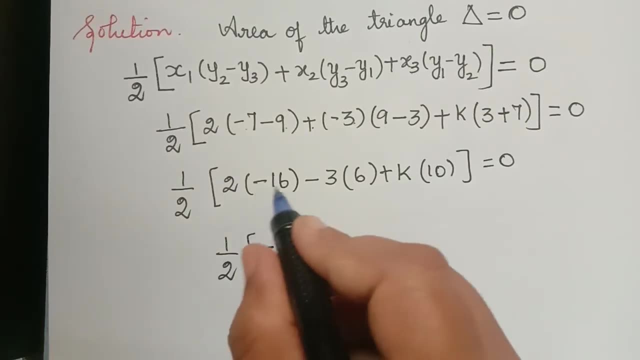 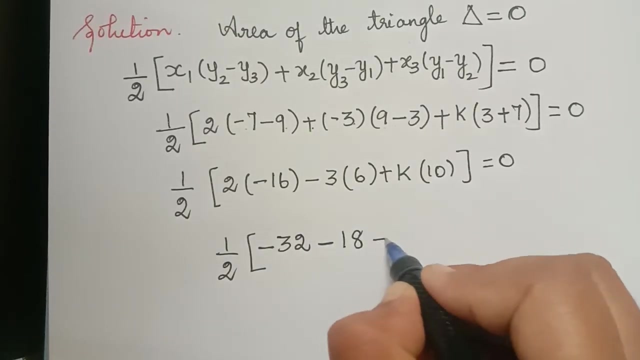 Now, further simplifying this, we get 1 by 2 of this will be 2 multiplied with minus 16, so we will have a negative sign. and 2 multiplied with 16 is 32 minus 3. 6 times is 18. plus k multiplied with 10 will give us 10k, and so this is equal to 0.. Now this 2, which is here: 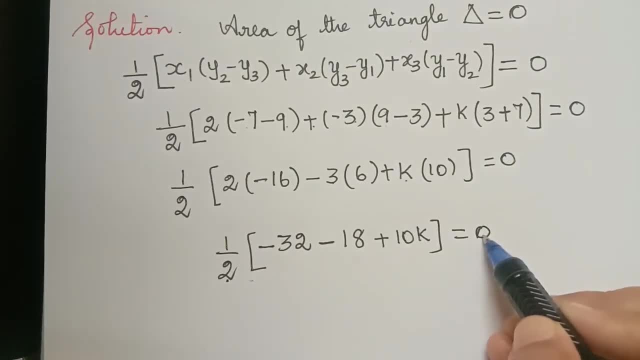 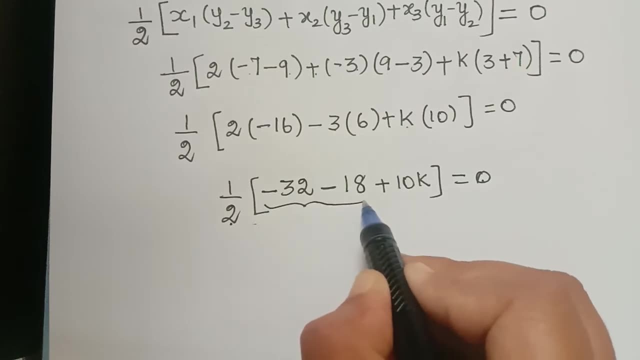 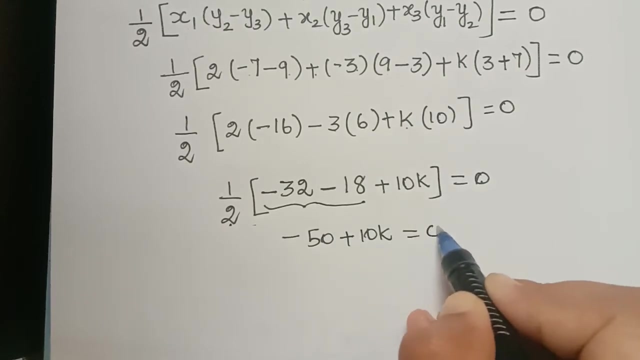 in the denominator it will be cross multiplied to this with this 0, and so 2 multiplied with 0 will be 0 only, and then minus 32 minus 18 is minus 50. So minus 50 plus 10k will be equal to 0, because this 2 gets multiplied with the 0, and so we get. 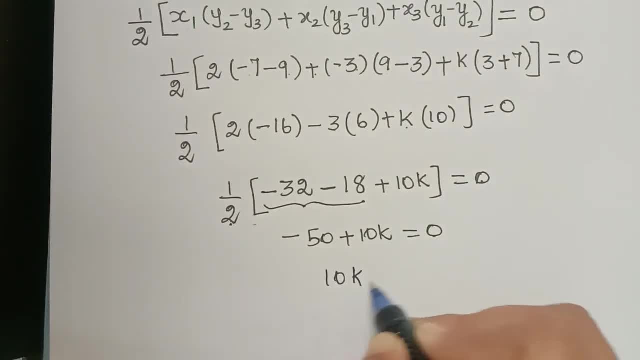 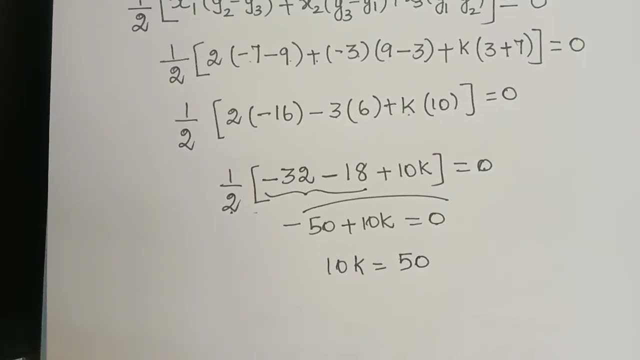 this as 0 itself, and so 10k will be equal to taking this minus 50 to the other side. it will become plus 50, so we will have 50, and so the value of k will be equal to 50 divided by 10. 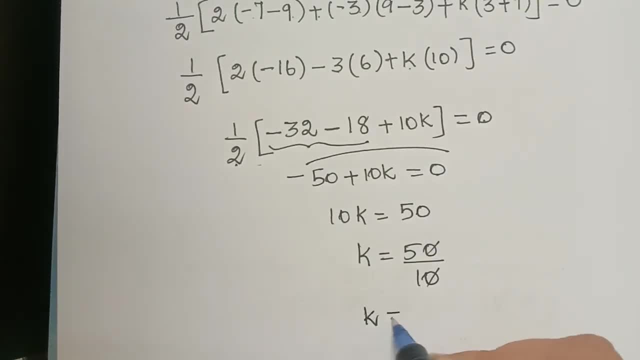 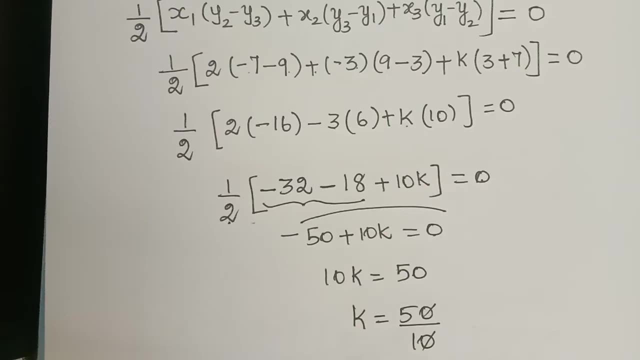 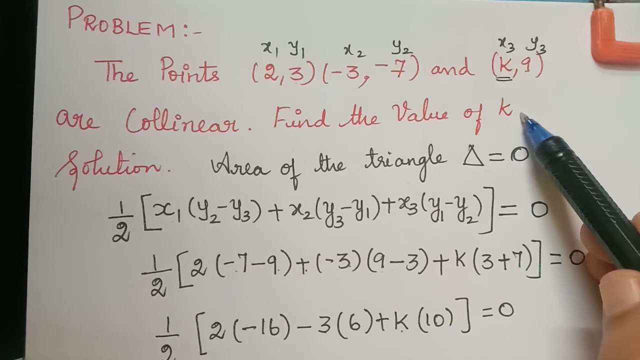 and so, cancelling this, we get k to be equal to 5 and so, therefore, the value of k is equal to 5. so we have obtained the required answer. Hope you have understood this problem. this is one of the significant problem in the examination point of view. so they may say they may give three points with one of the coordinators unknown. 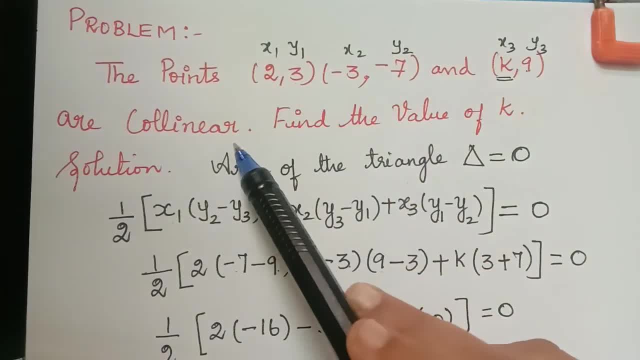 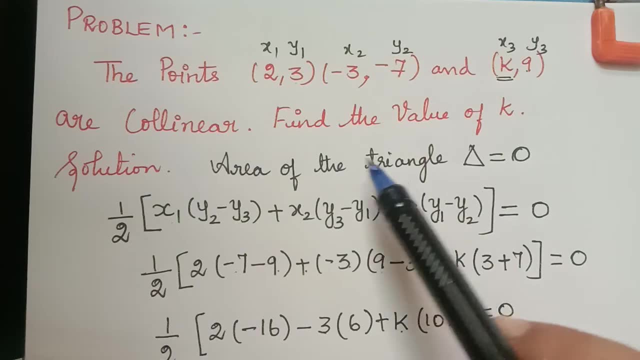 and they may give the condition that the three points are collinear and they will ask you to find the value of that unknown. so in that case we know that the if three points are collinears in the area of the triangle will be equal to 0.. 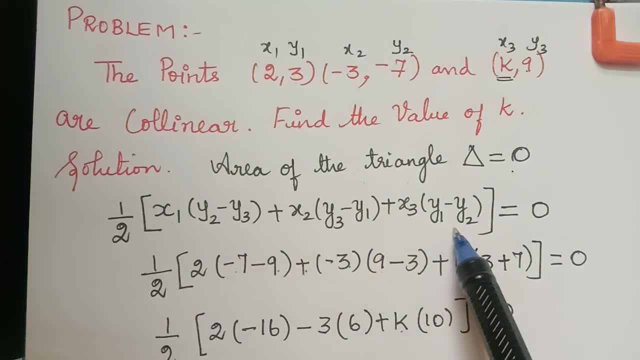 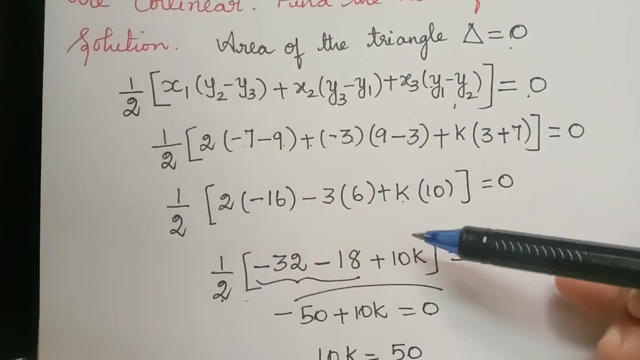 0, and so we are substituting the formula of the area of the triangle here which is equated to 0, and substituting each of the coordinates. we simplify it and we find the value of k. So this is how we solve this kind of problem. Thank you.